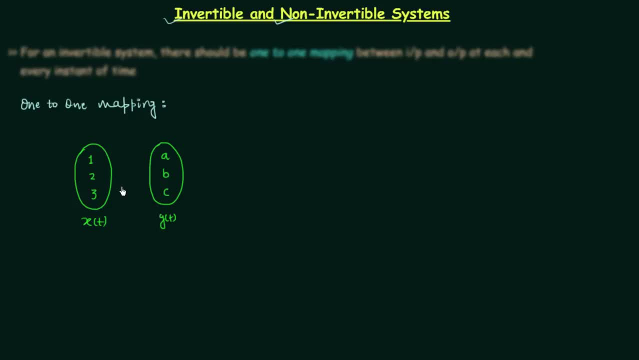 all the three values of input will produce three distinct values of output. Let's say, when xt is equal to 1, the output yt is equal to b, When xt is equal to 2, the output yt is equal to a, And when xt is equal to 3, output yt is equal to c. So you can clearly see all the three. 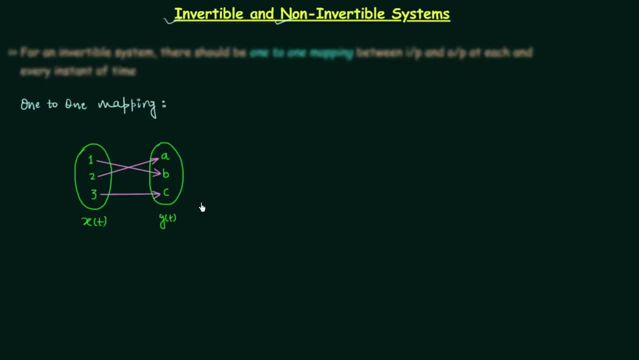 values of input are producing three distinct values of output, So this particular mapping is known as one-to-one mapping. And now we will understand what do we mean by many-to-one mapping. In case of many-to-one mapping, two or more distinct possible values of input will produce 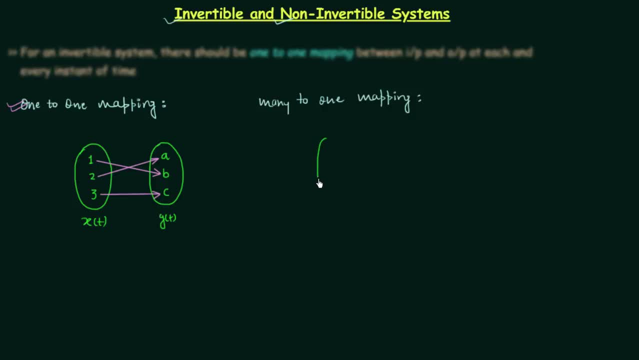 the same output. Let's understand this by the help of one example. In this example, this is the set of possible values of input. So let's say we have two different values of input. We have two different values of input xt. Let's say the values are 2,, 4, and 6.. And now I will draw the 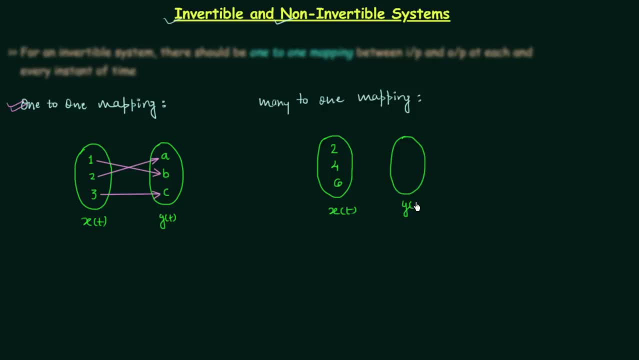 set of possible values of output yt. Let's say the outputs are a and b. Now this two here will produce the output yt equal to b. This four here will produce the output equal to a And this one here will produce the output equal to b. So you can clearly see when xt is equal to 2,. 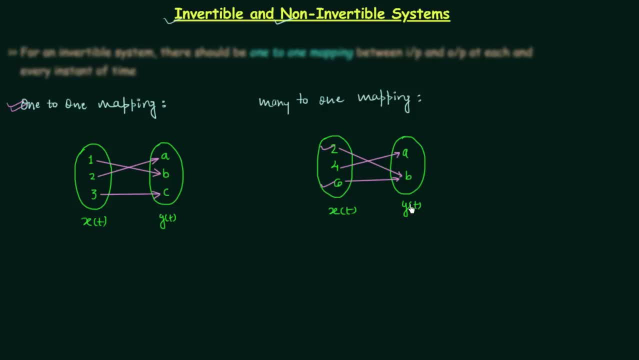 the output is equal to b. When xt is equal to 6, the output is again equal to b. So for two distinct possible values of input, the output is same, that is, b. So this particular case is known as many-to-one mapping. There are many inputs producing the same output And this is the mapping. 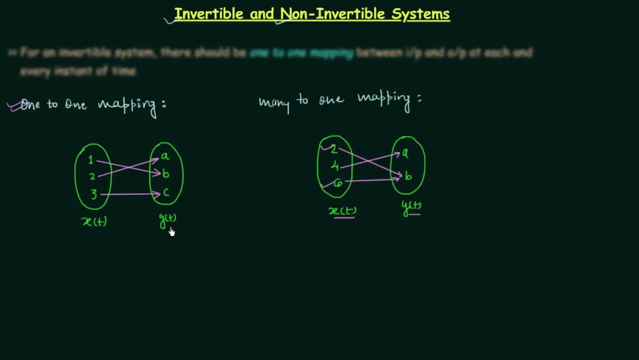 between input and output, And this is the same output And this is the same output, And this is the. Here also we have the mapping between input and output. So we are done with one to one mapping and many to one mapping, and now we can understand. 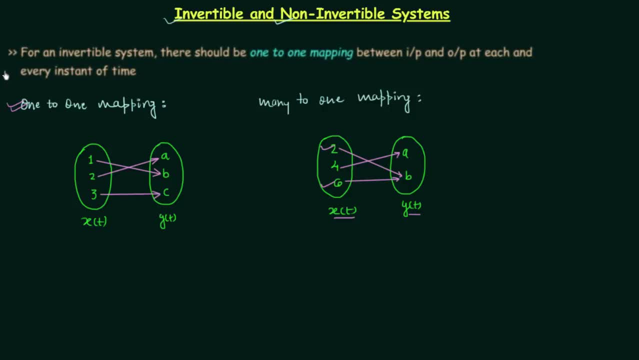 the definition of invertible systems. You can see the definition on your screen. For an invertible system, there should be one to one mapping between input and output at each and every instant of time. So in case of invertible systems, there should be one to one mapping between input and output. 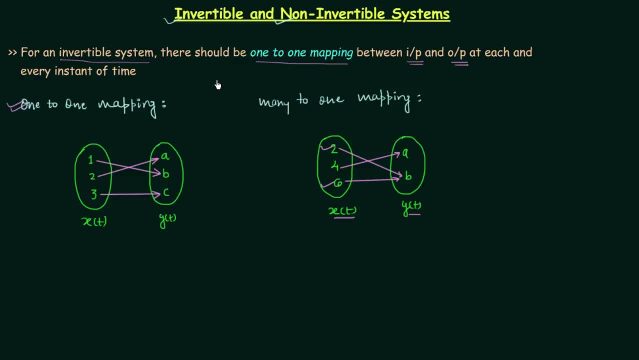 at each and every instant of time. On the other hand, in case of non-invertible systems, instead of one to one mapping, we have many to one mapping. Let's take two examples to understand this. In example number one we have the system relationship like this: yt equal to xt square, and we will 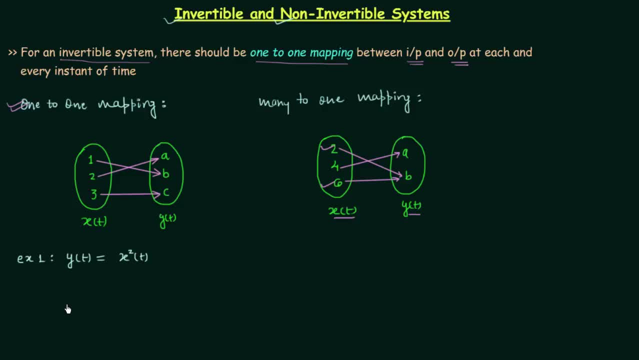 check this. Let's check whether they follow the one to one mapping or many to one mapping. For this I will make a table and in this table the first column is for the input and the second column is for the output, And I will choose different values of xt and we will calculate the corresponding yt. 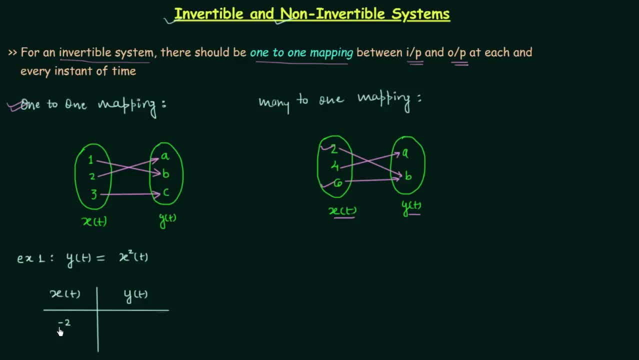 Let's say xt is equal to minus two. When you put minus two here, you will have minus two square. therefore yt will be four. Now let's put xt equal to two. When you put two here again, you will have yt equal to four. 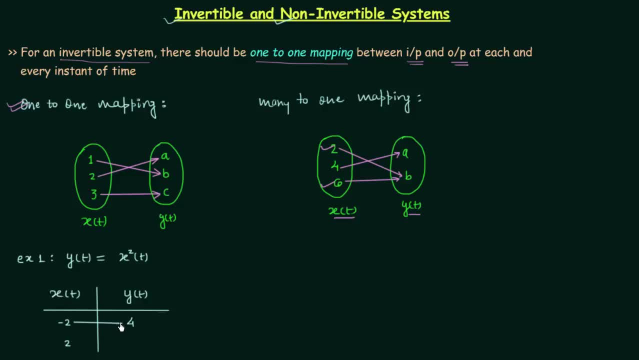 So we have many to one mapping. This minus two is producing four and this plus two is also producing four. So it is case of many to one mapping and as there is many to one mapping, this system is non-invertible. Let's check. 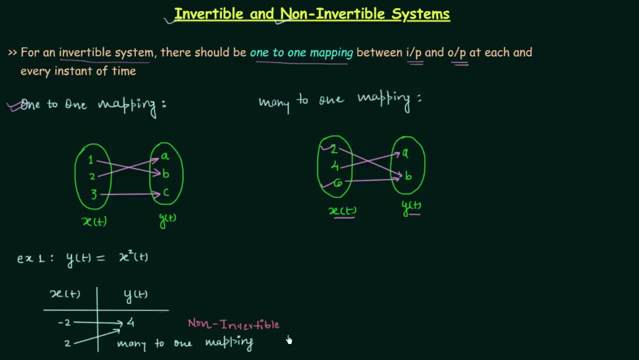 Let's check. This is non-invertible. So this is our answer. Now let's take example number two. In the second example, Output yt is equal to xt plus two. Again, we will follow the same steps. First, we will make the column for the input. 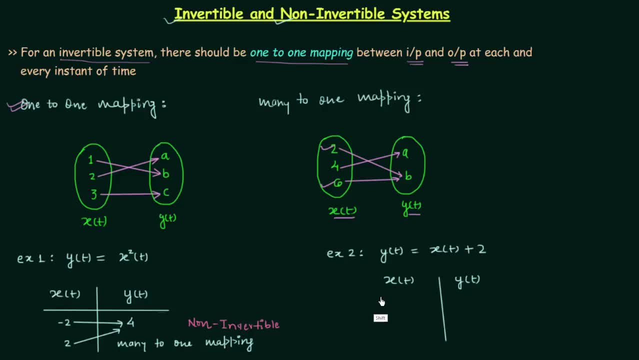 Then will make the column for the output And we will choose some values of input And we will calculate the corresponding output. Let's check. Let's say xt is equal to 0. This will give us yt equal to 2.. Let's make xt equal to 1, yt will be. 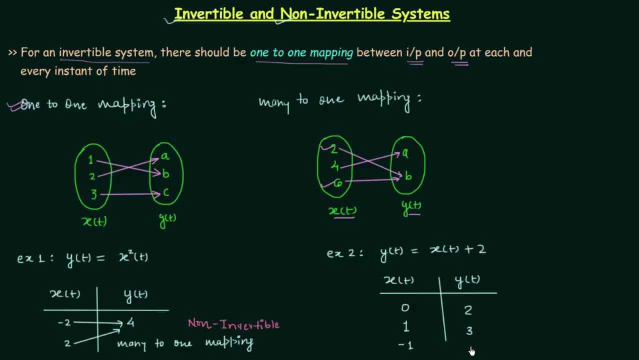 3. xt equal to minus 1, yt will be 1.. So for different possible values of input we have different values of output. So it is the case of one to one mapping. 0 is giving us 2, 1 is giving. 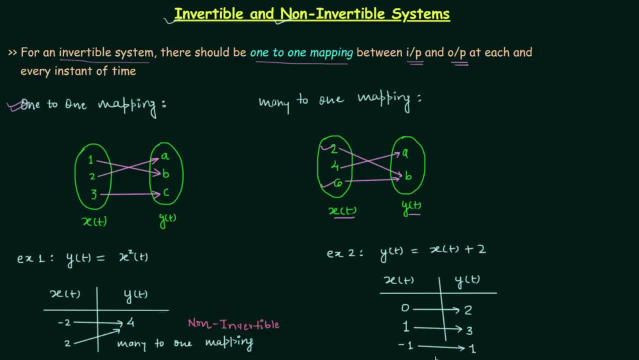 us 3, minus 1 is giving us 1.. And in the same way, if you check the other values of input, you will get distinct values of output. So this case is the case of one to one mapping And therefore 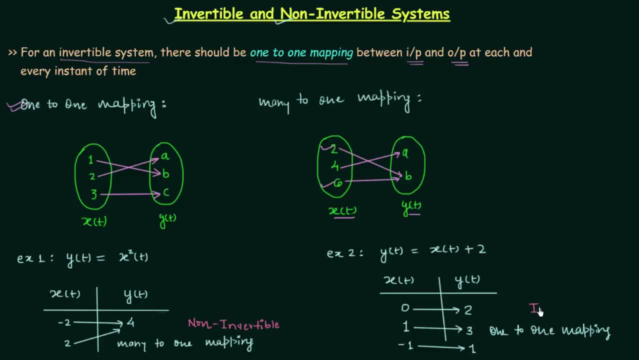 we can say that the system is invertible. So I hope you now understand what do we mean by invertible and non invertible systems And what is one to one mapping and many to one mapping. Now we will move to the next part. 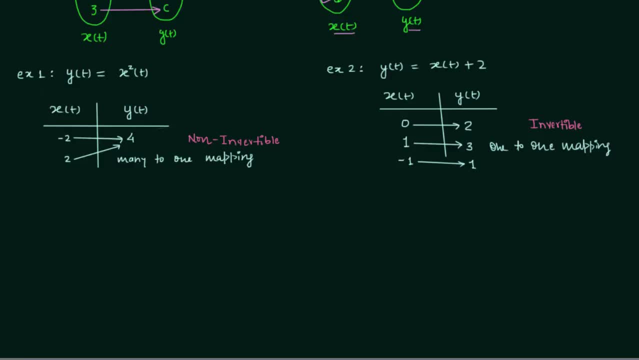 of this lecture in which we will discuss one important property of invertible systems. The first box here represents the invertible system And the second box here represents the inverse system of this invertible system, and they are cascaded together, So we have a composite system. 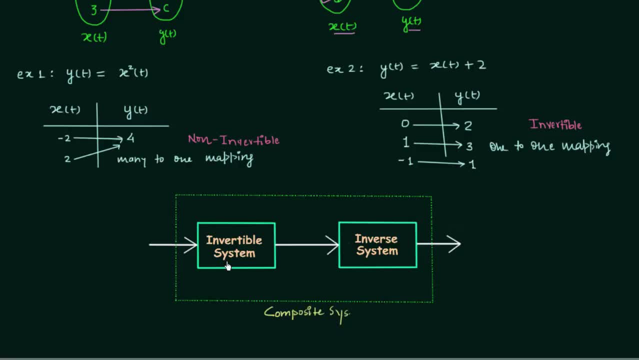 which we have obtained by cascading invertible system with its inverse system. When an invertible system is cascaded with its inverse system, then the overall gain of composite system will be equal to unity. Let's say xt is the input to the invertible system and the system is producing the output, yt. And when this 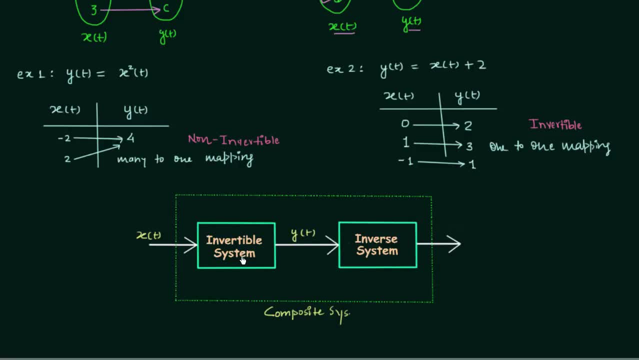 output, yt, is subjected to the inverse system of this particular invertible system. the output we get is equal to xt And when you calculate the gain it will be equal to unity, because output is same as the input. So the composite system is having the gain. let's say the gain is hs for 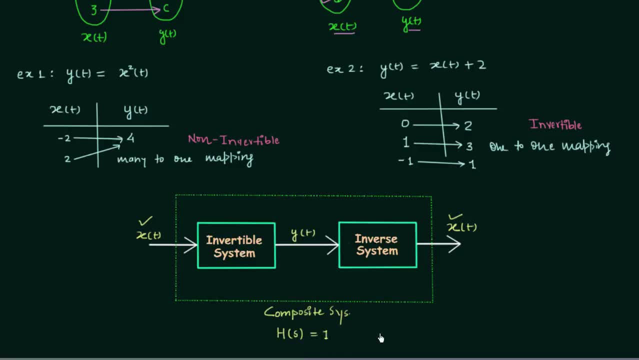 composite system it will be equal to one. let's say the gain of invertible system is h, subscript i s and the gain of inverse system is h2 s. Then we already know from the control systems: hs will be equal to h i s multiplied with h2 s And.